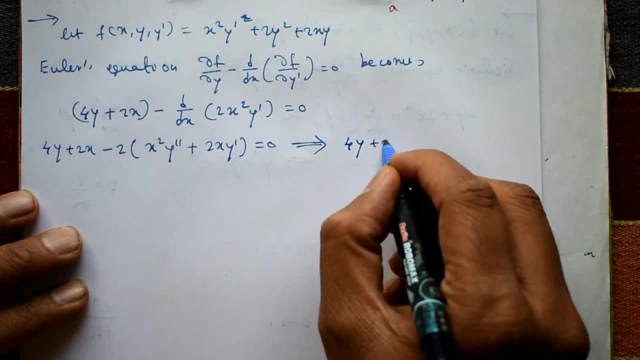 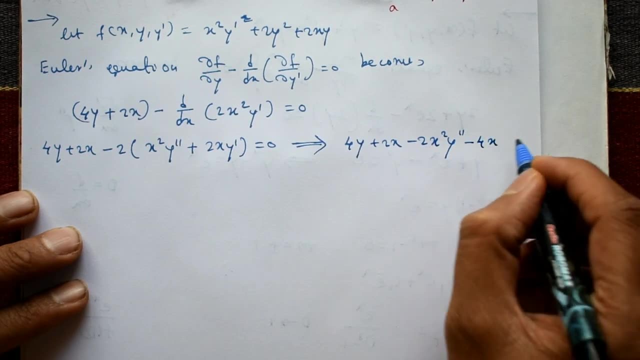 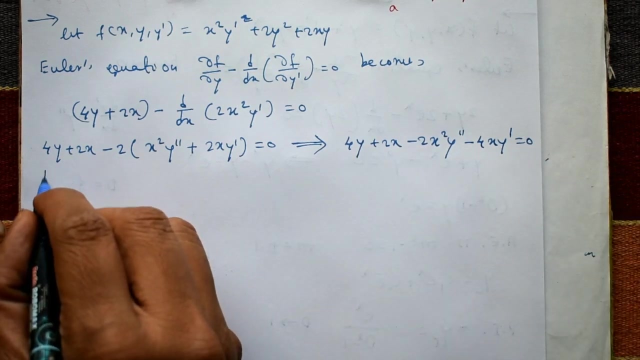 Ok, Now next step is 4y plus 2x. open this bracket minus 2x. square y, double dash, Again minus 4xy, dash equal to 0.. Ok Now in this equation is dividing by 2.. Dividing by- I will take better- is minus 2.. 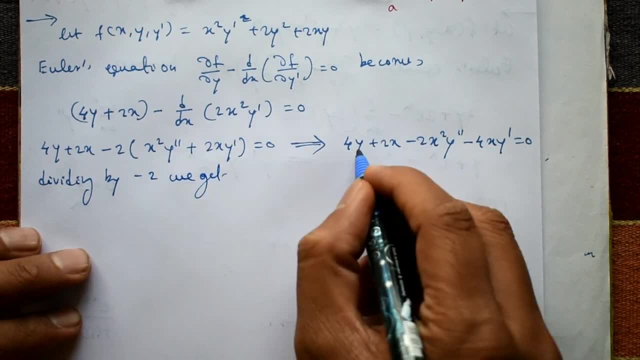 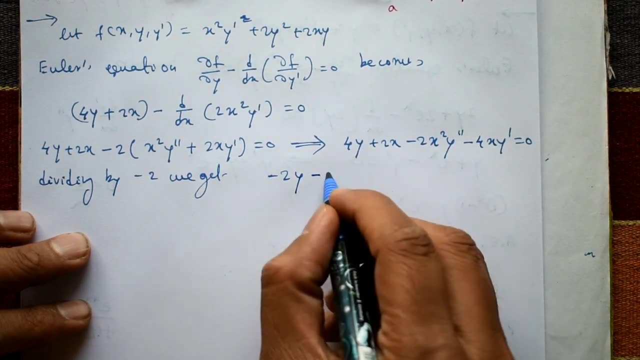 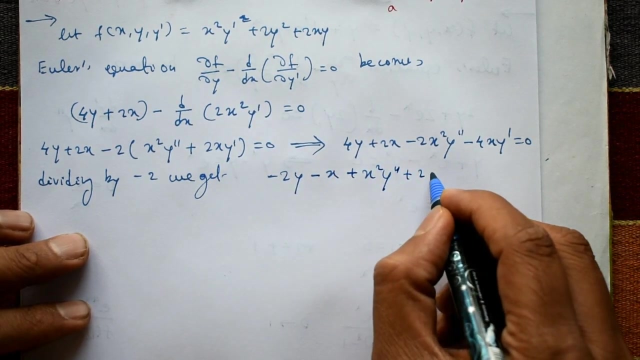 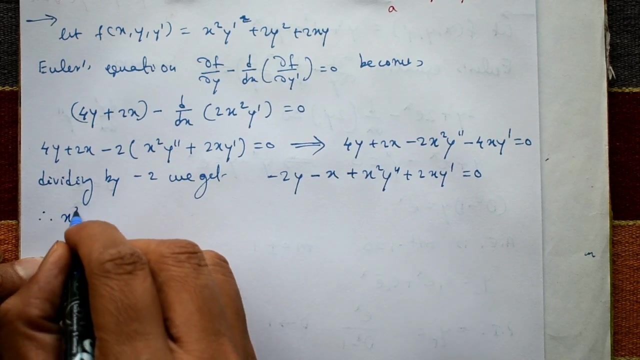 Minus 2. we get. dividing by minus 2 means this is minus 2y, minus x and plus x square y double dash and plus 2xy dash equal to 0.. Ok Now, therefore, alright, order wise, this is x square y double dash, first term. 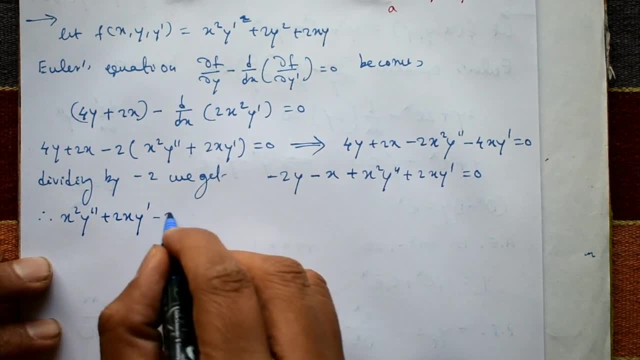 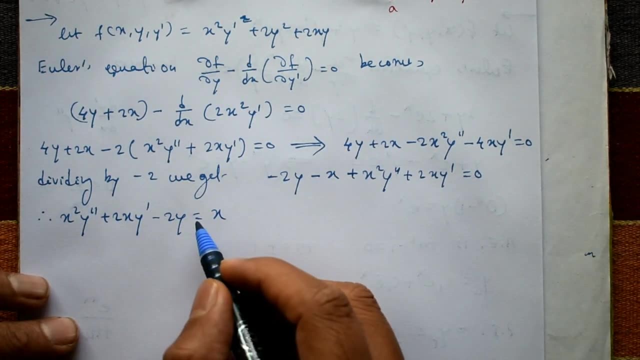 This is second term. 2xy dash- This is minus 2y- is equal to shift right hand side. we get plus x. Now see this equation. Now, this equation is a Cauchy's linear equation. This is equation number 1.. 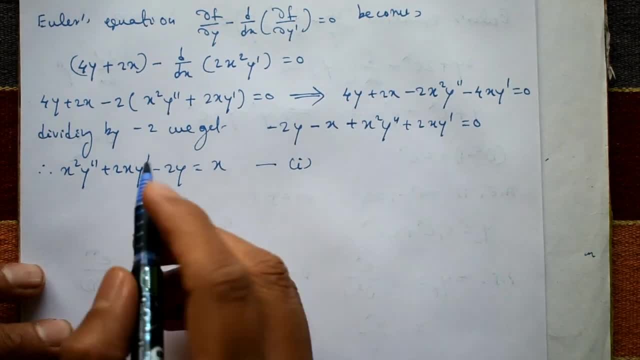 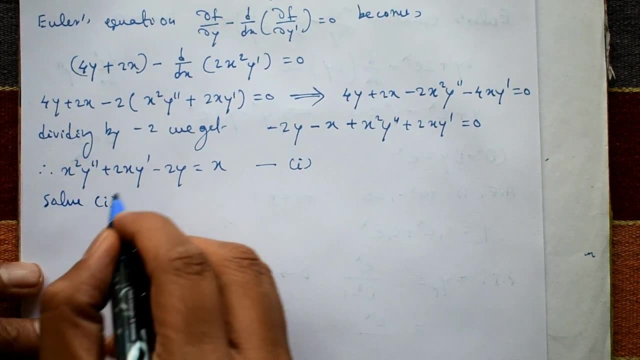 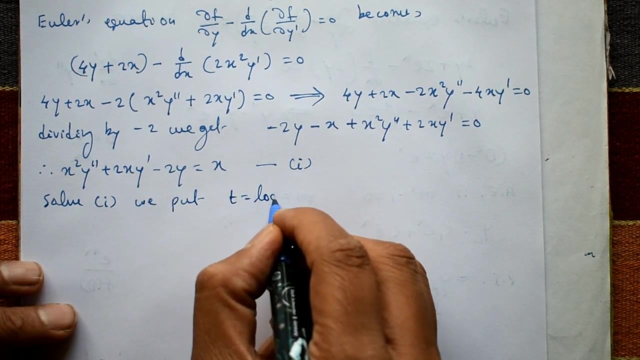 Ok, Cauchy's linear equation. You know the method of Cauchy's linear equation. Now solve equation number 1 means this equation We put. this is Cauchy's linear equation. Put t is equal to log x or x is equal to e. raise to t. 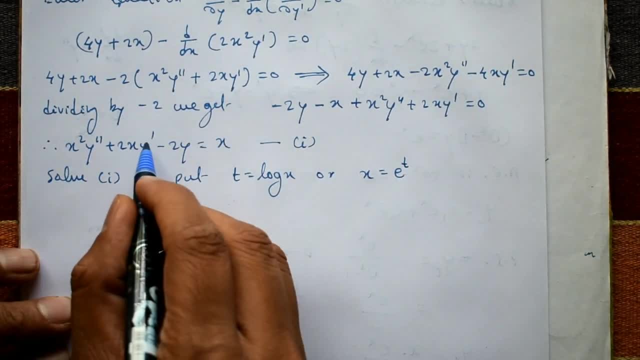 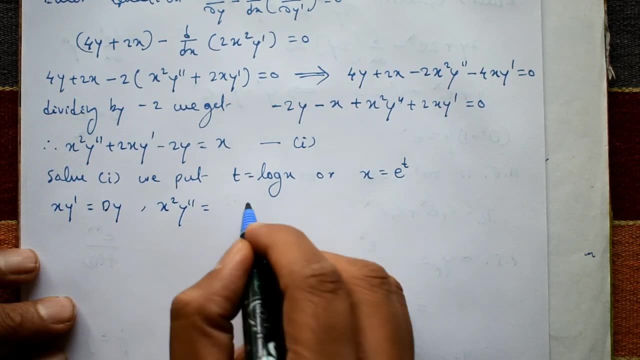 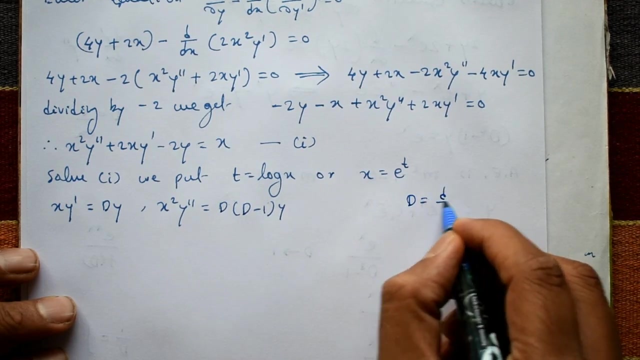 This is very simple Now: x square y double dash and xy dash. xy dash is d into y and x square y double dash is d into d minus 1 into y. Ok, d minus 1 into y. So in this equation d stand d by dt. 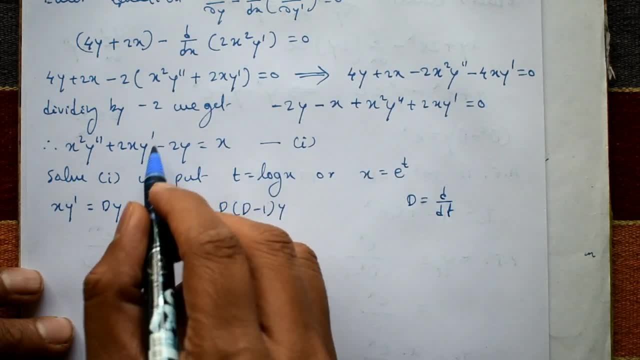 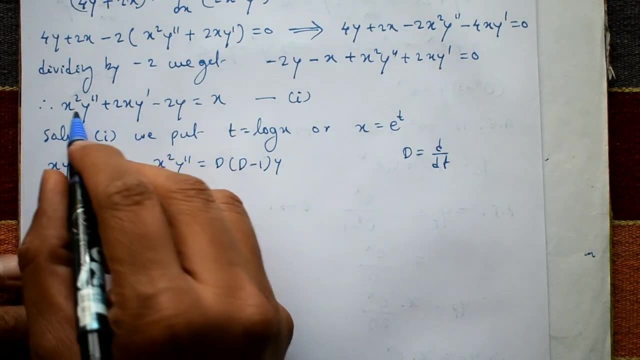 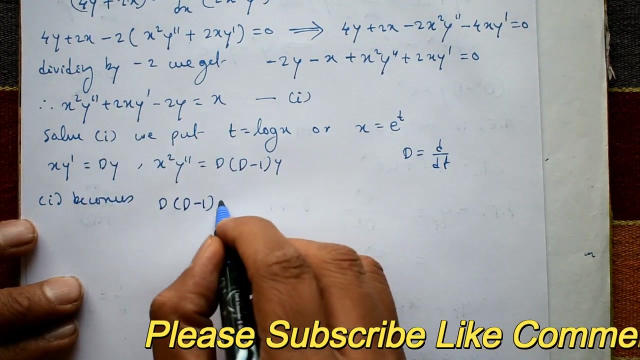 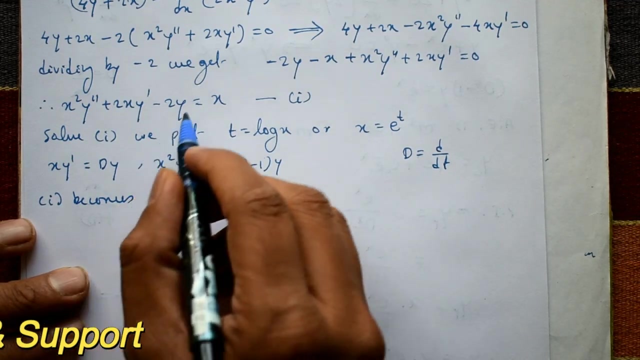 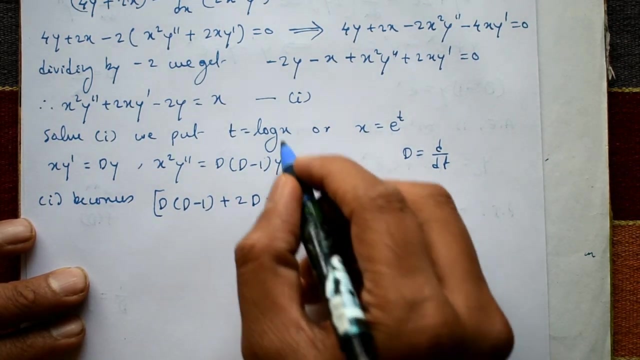 Ok, Now these result are substitute in equation number 1.. Equation number 1 becomes: x square y. double dash is d into d minus 1 plus 2xy dash is a d minus 2 and y is a common. take y is outside, sorry- into y that is equal to x. 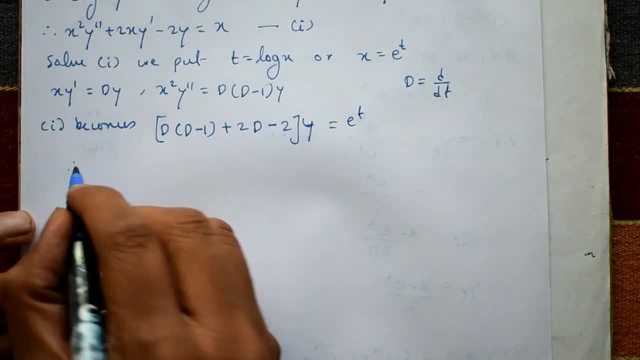 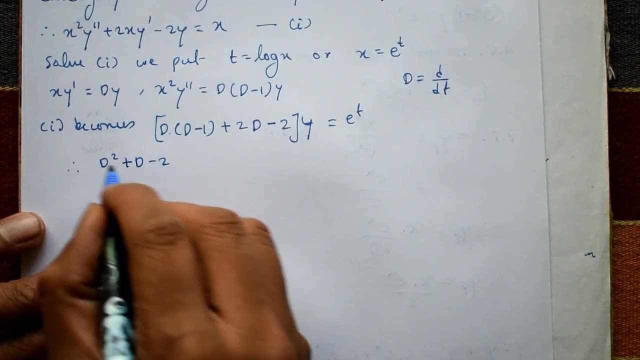 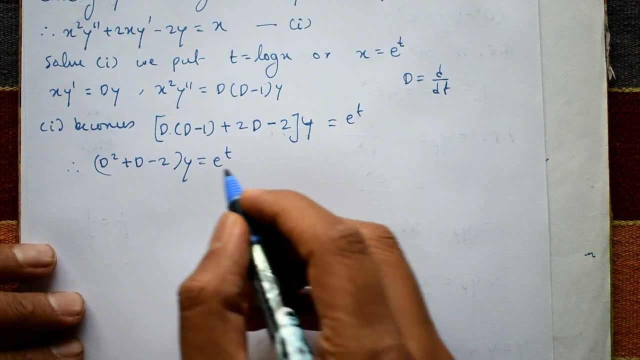 x means e. raise to t. Ok Now. therefore, now it is a d square minus d plus 2d, plus d only, and minus 2 into y is equal to e. raise to t. Now find the y solution Now. first we need a auxiliary equation. 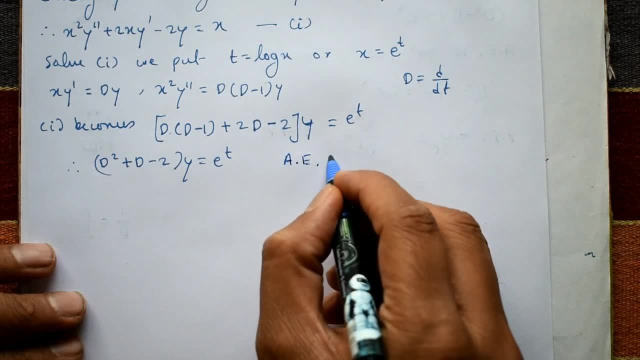 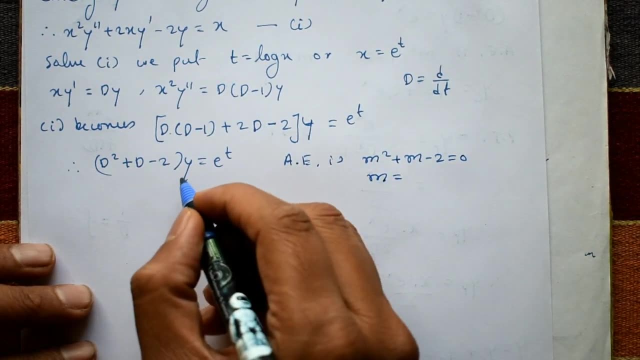 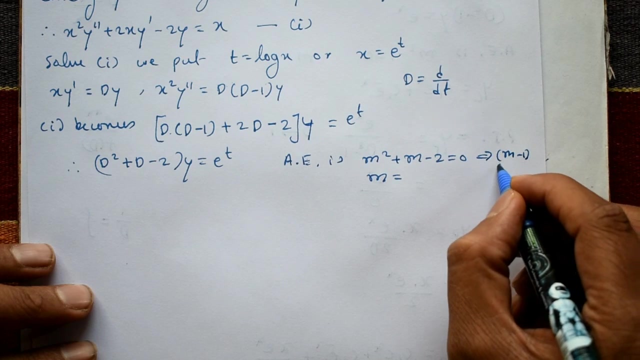 Ok Now auxiliary equation is now: this: is a m square plus m minus 2, equal to 0, and m is equal to factorization. You get m. this is like this: m minus 1 into m plus 2, m plus 2: that equal to 0.. 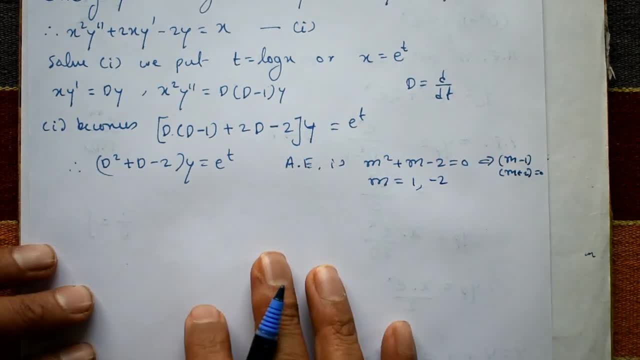 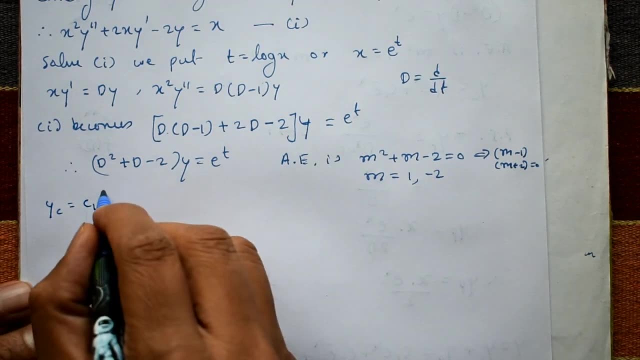 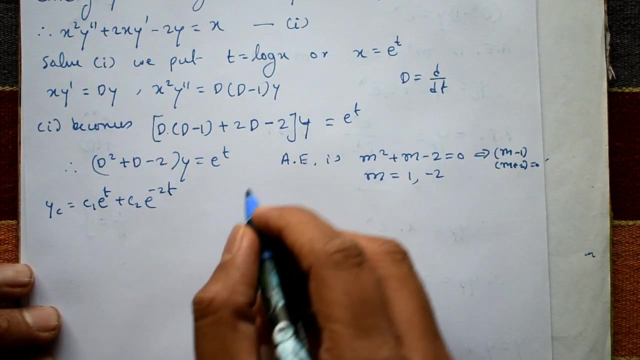 Factorization you get: m is equal to plus 1 and m is equal to minus 2.. Ok Now, complementary function is: roots are unequal, means different: c1 e raise to t plus c2 e raise to minus 2t. Ok Now, next we need a particular integral. 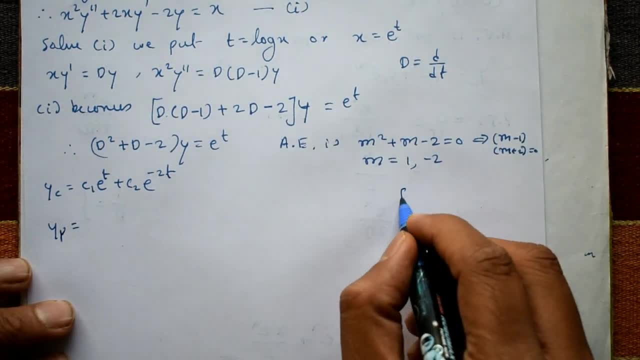 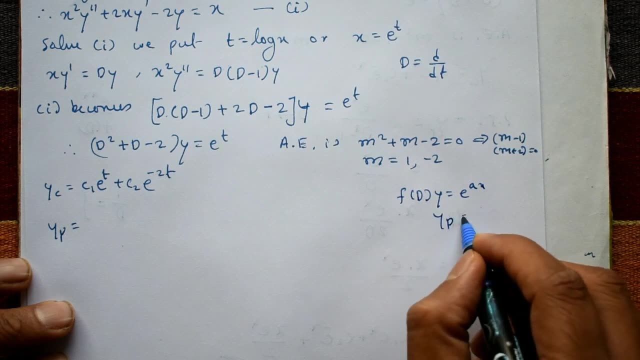 Particular integral. Ok, Now, generally particular integral is: a f of d into y is equal to e. raise to x. Now go to the particular integral: e raise to ax upon f of d. Now, taking right hand side, that is, e raise to t upon f of d means now this is a d square plus d minus 2.. 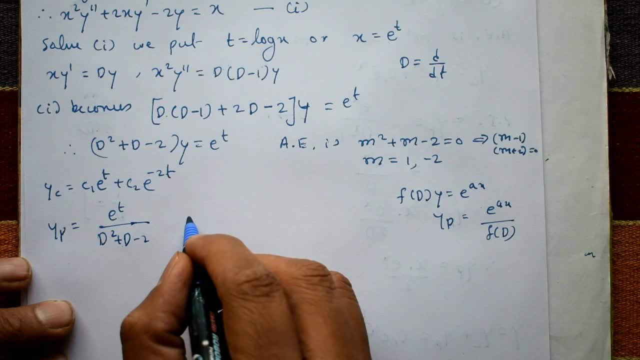 Now particular integral. Now this type taking d is equal to a. Ok, e raise to a t. a means 1.. d is equal to 1.. Put d is equal to 1. we get e raise to t is equal to denominator 1 plus 1 minus 2, that is 0.. 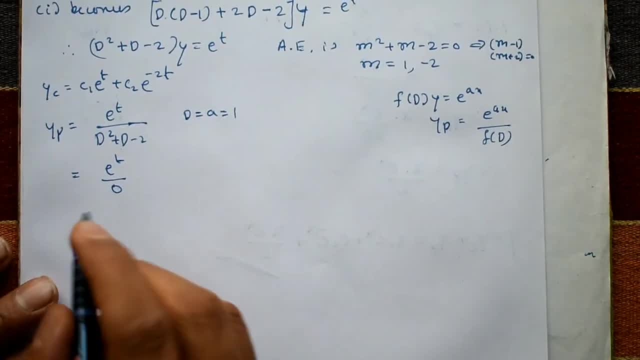 Denominator is 0.. So that m, Now particular integral, multiply by t in numerator and e raise to t upon difference. say this one: 2d plus 1.. Difference: say this one: this is 0.. 2d plus 1.. 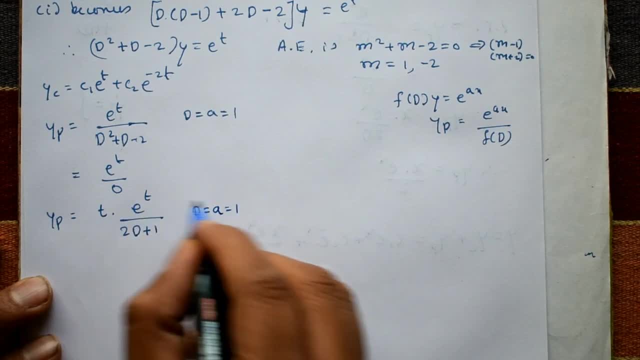 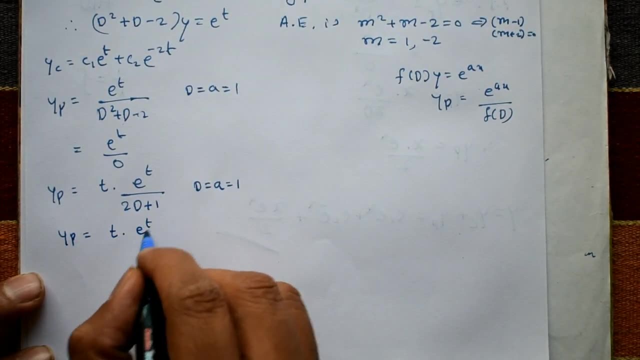 Again same procedure. d is equal to a, a means 1.. That means d is equal to 1. only Now, particular integral is t into e. raise to t by 2 plus 1 is a 3.. Ok, Now solution is general, solution is: